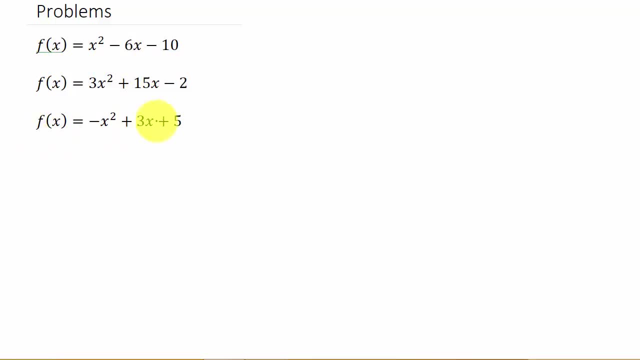 This will be in the second video, example two, And this one will be the third example in the third video. Alright, so you can go to whichever video you need, Alright, so? So let's go ahead and get started. 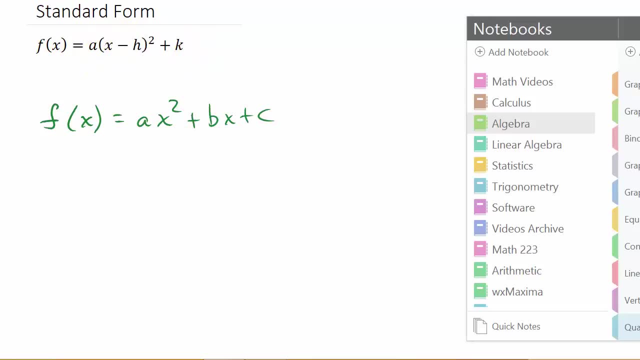 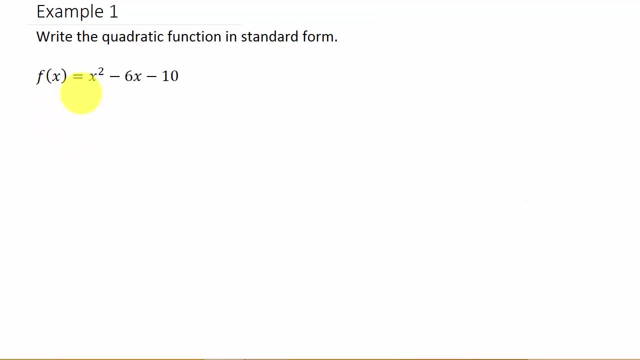 Okay, it's going to be in this form and we're going to convert it to this standard form. Alright, so let's look at example one. Alright, so we have: f of x is equal to x squared minus 6x minus 10.. 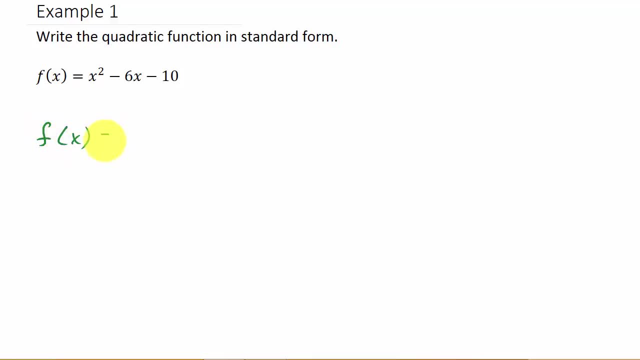 Alright, so what we want to do is we want to take f of x equals x squared minus 6x, And we want to separate this from the constant, And we want to leave a little space here, minus 10.. Okay, so what we're going to do is complete the square on it. 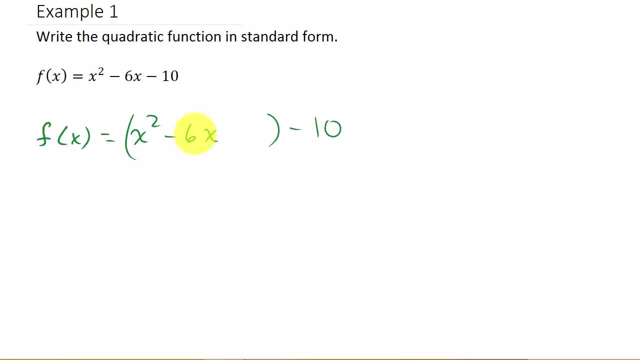 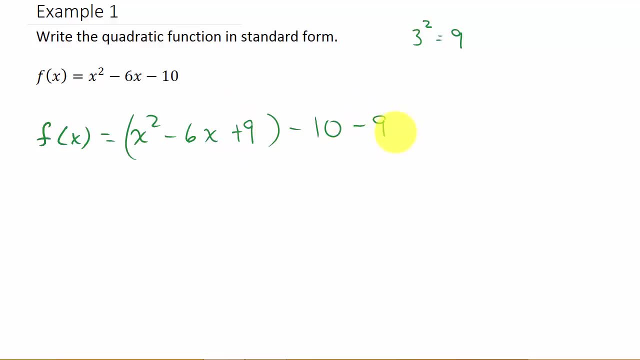 And since we added 9 here, we have to subtract 9 here. Okay, so basically what we did is, if you look at these two numbers here, 9 minus 9, basically what we did is we added 0.. Okay, so by adding 0, we don't change the problem up. 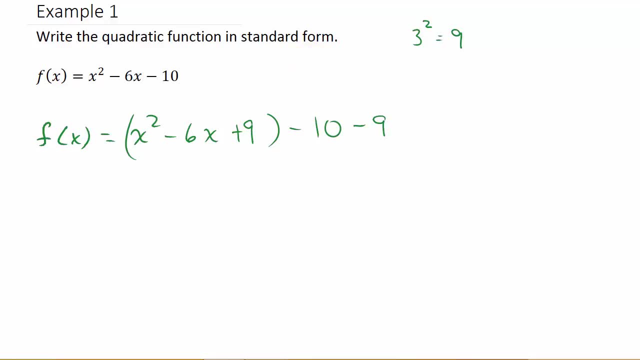 Okay, alright, Alright. so now we have We have f of x is equal to. Now this thing is going to factor. Okay, this is what we call a perfect square trinomial. So we know it's going to factor into this. 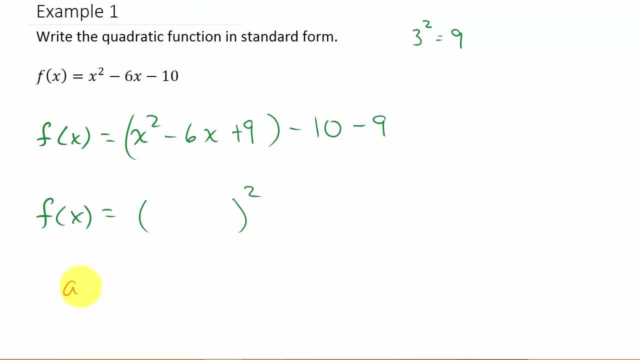 Okay, it's Remember it's in one of these forms here: A x squared. I'm sorry, It's in this form: x squared minus 2xy, y plus y squared. That's the form this is in And it factors into this.